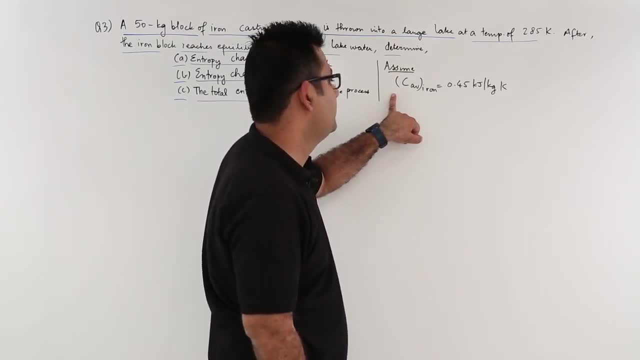 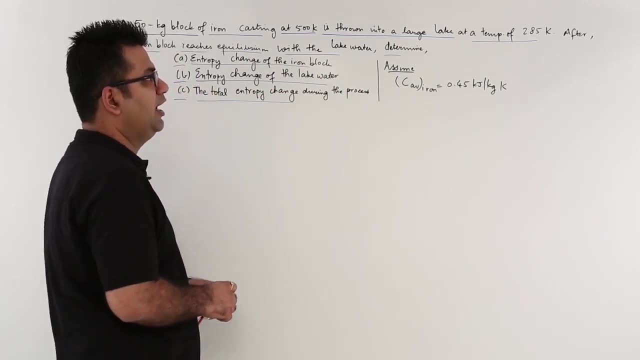 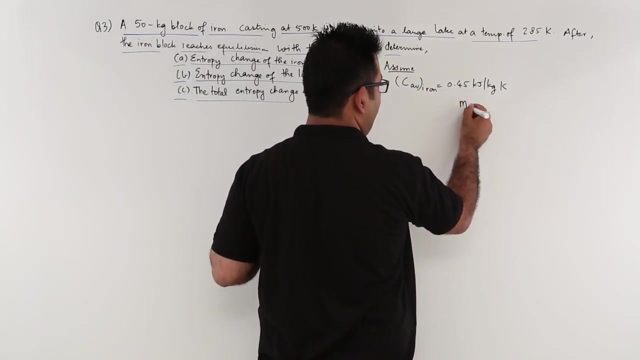 We need to assume the average. you can say the specific heat capacity of iron as 0.45 kJ per kg Kelvin. So let's start by writing down the given. That's the very first step. you should always do So. the mass of the iron block: this is 50 kg. 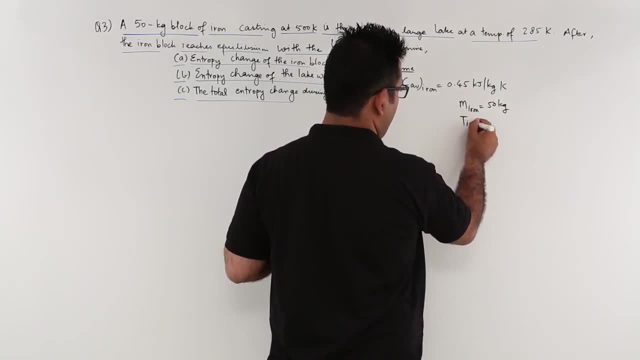 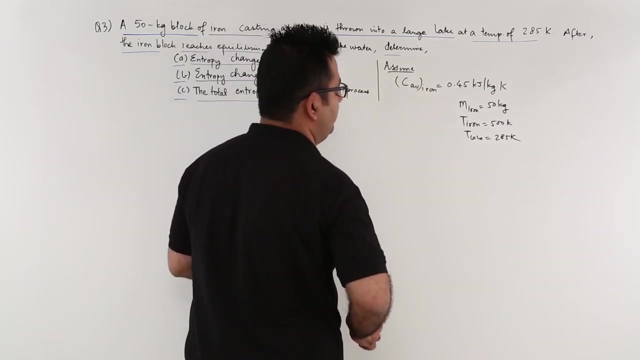 The temperature of the iron block is 500 Kelvin and the temperature of lake is 285 Kelvin. So the very first thing is to find out: is it delta is for iron? So the first thing is to find out: is it delta is for iron? 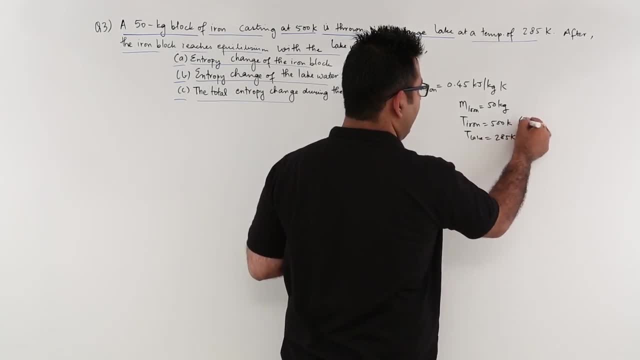 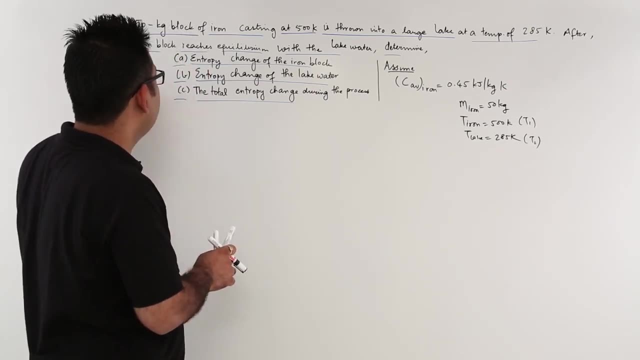 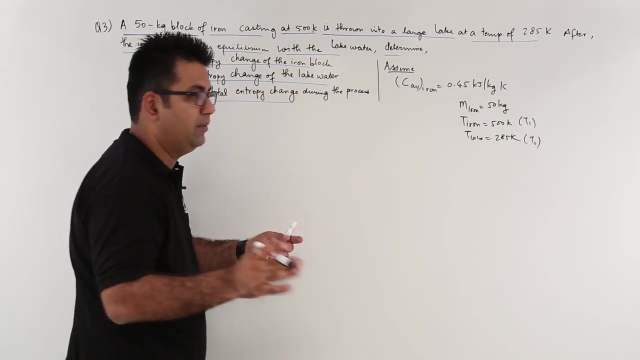 So we can assume that this is T1 and this is T2 with respect to iron, because, you know, ultimately this is reaching the equilibrium. So the iron and lake, they have no delta T, so there is no heat flow at that. you know, equilibrium. 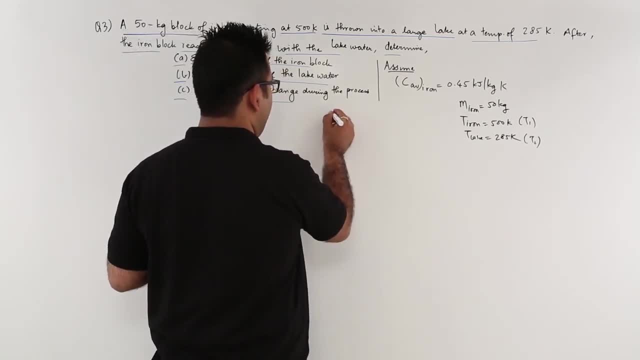 But you know, let's find out: delta S for iron. Delta S for iron that is equal to M into C A V. Delta S for iron that is equal to M into C A V, into natural log of T2 by T1.. 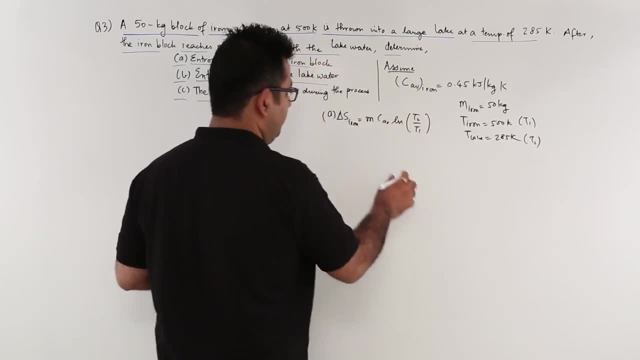 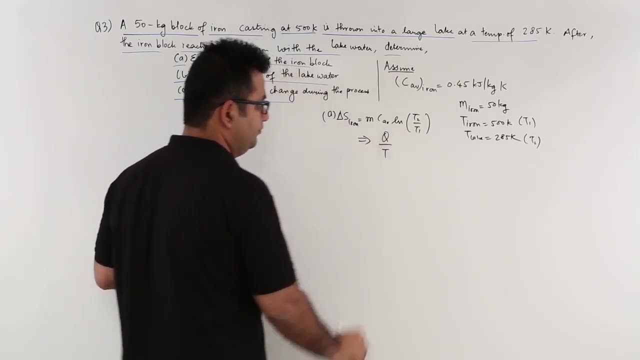 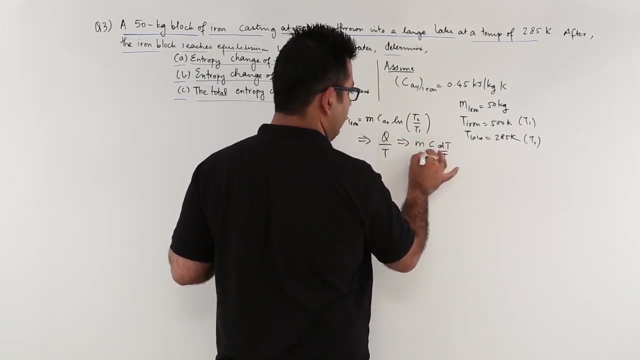 Now, how did we get over here? See, this is nothing but. or you can say Q upon T, Isn't it? Now, what is Q? Q is MC DT. If you integrate this, you get MC log T2 by T1.. 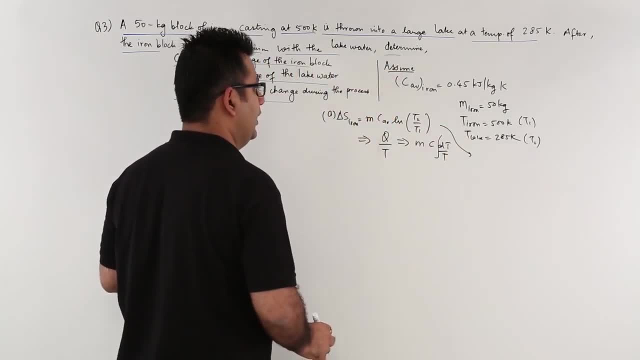 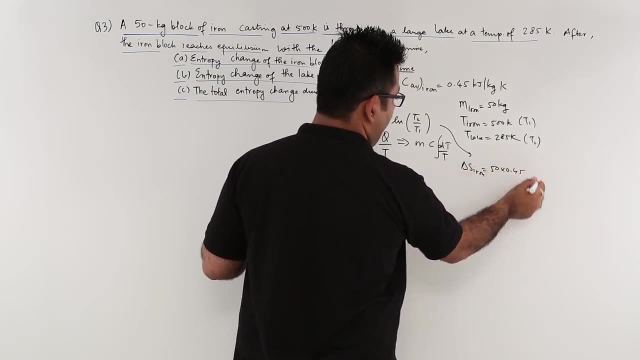 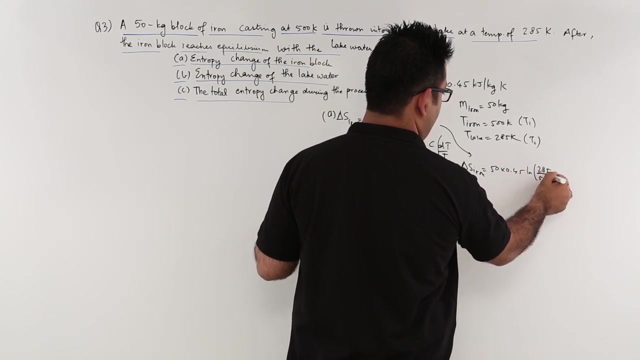 So let's continue with the calculation. So this becomes Iron. this is 50 into 0.45, into log 285 by 500.. Okay, So it will be a negative quantity because iron is, as it is, losing heat, so the entropy would go down. 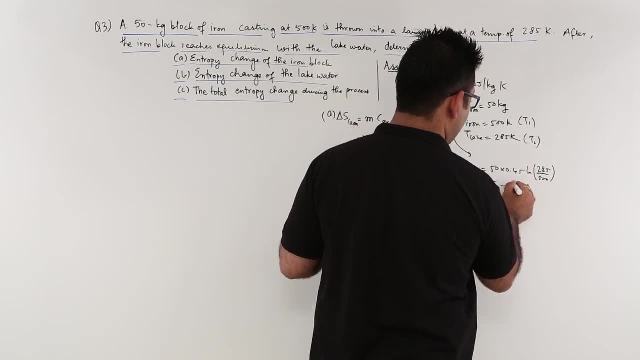 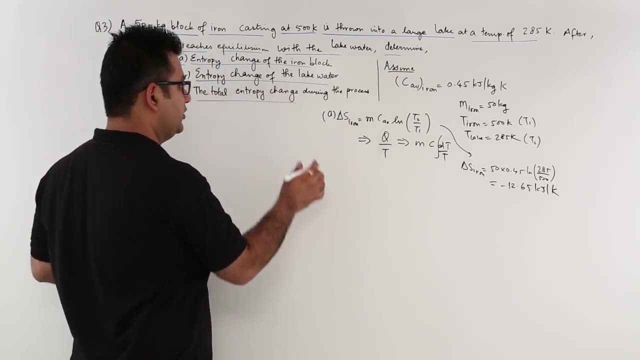 So it will be a negative value. So this will be equal to minus 12.65 kilojoules per Kelvin. Okay, Okay. So the second part of the question is: what is the entropy change for lake water? 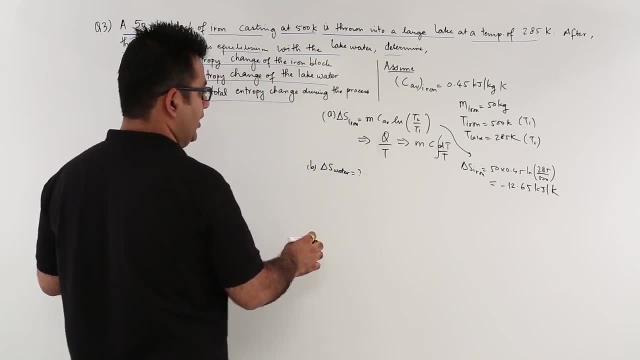 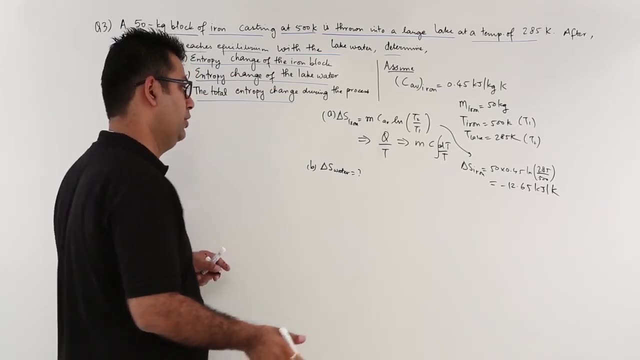 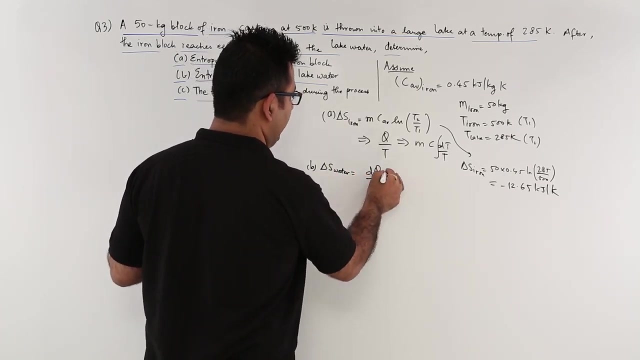 Okay, So for lake water you can say the amount of heat lost by iron is equal to the amount of heat gained by lake water. So I can still use DQ by T. So this would give you first of all, let's find out- DQ. 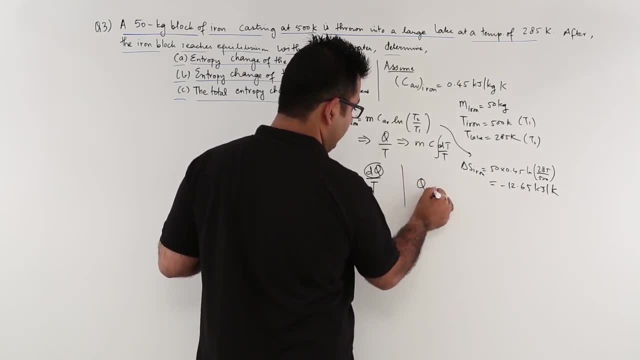 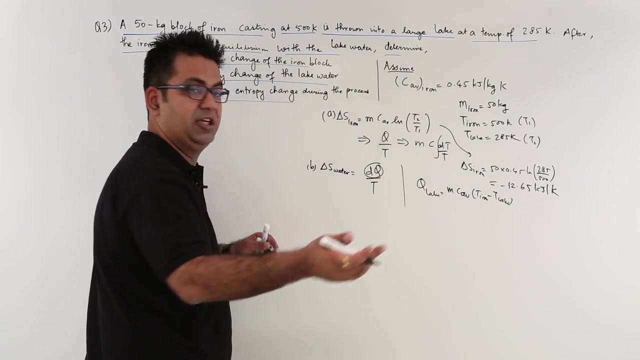 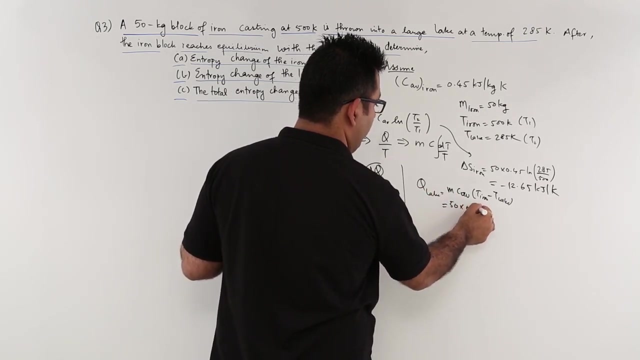 Okay, So Q lake is equal to M into CAV, into T iron minus T lake, So that is the amount of heat lost by the iron block. So this will be equal to 50 into 0.45, into 500. 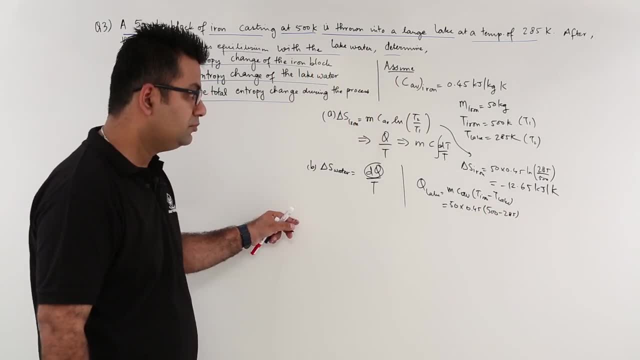 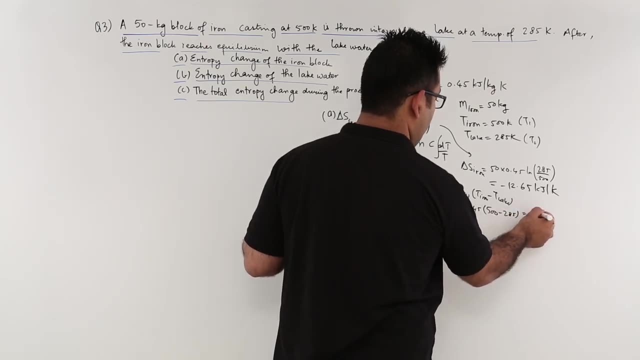 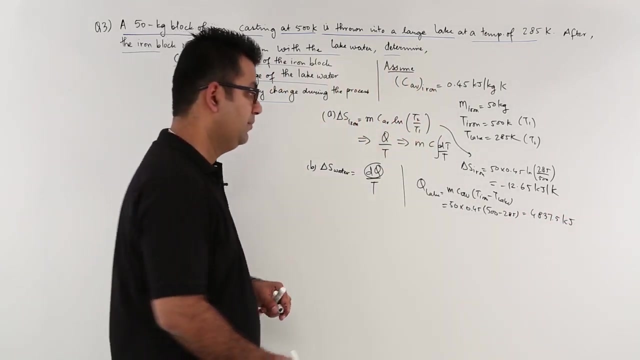 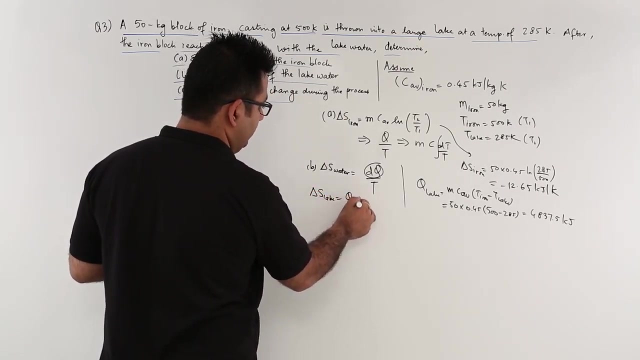 Okay, Minus 285.. So the answer of the heat gained by the lake water would be around 4837.5 kilojoules. Okay, So when you put this over here, so this would become Q lake upon T lake. 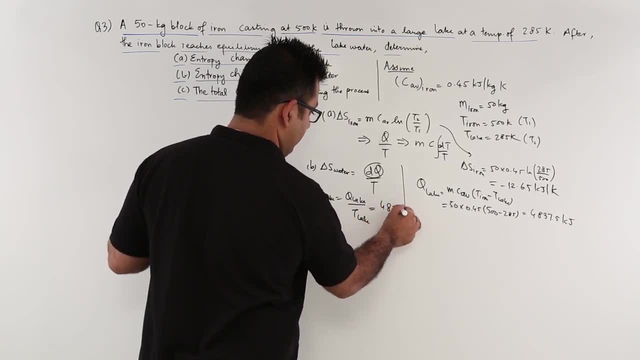 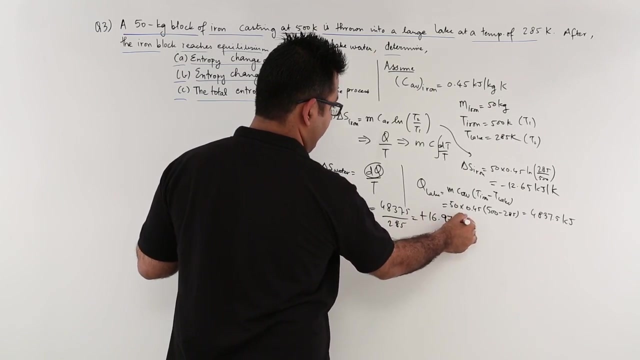 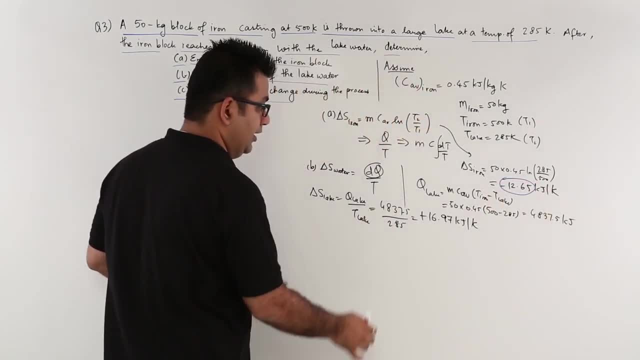 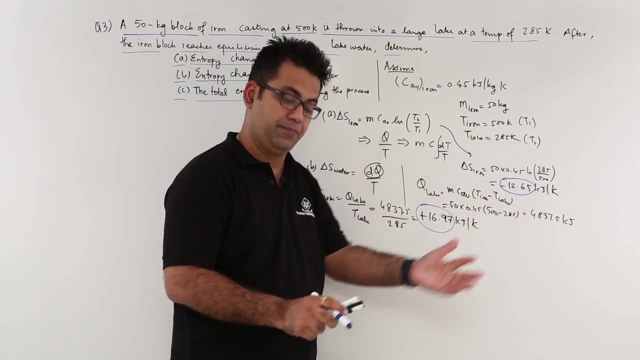 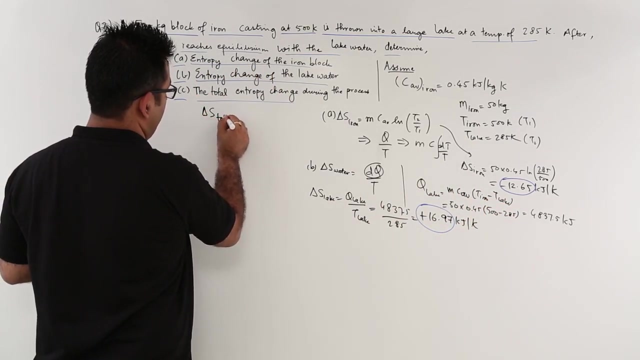 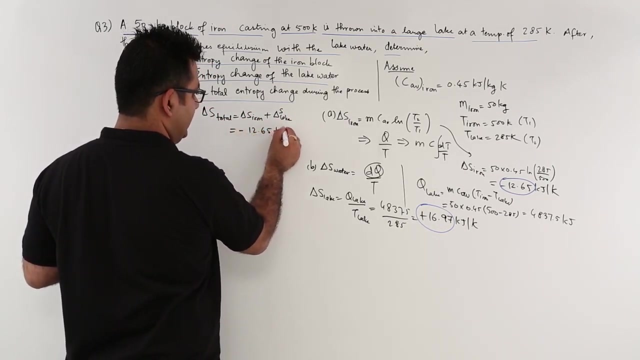 first value is the delta s for iron, and now you have delta s for lake water. the total entropy change would be sum of these two things, so i can write down that the total entropy change is equal to delta s iron plus delta s lake. so this becomes minus 12.65, plus 16.97. 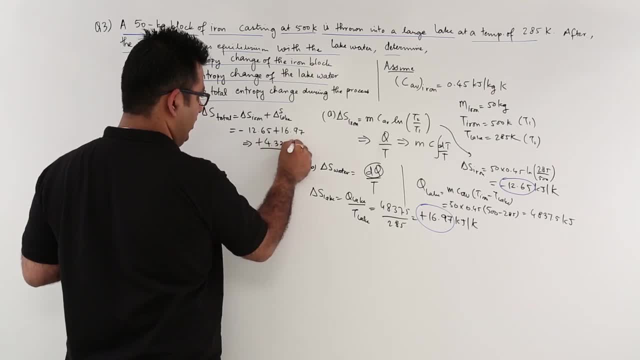 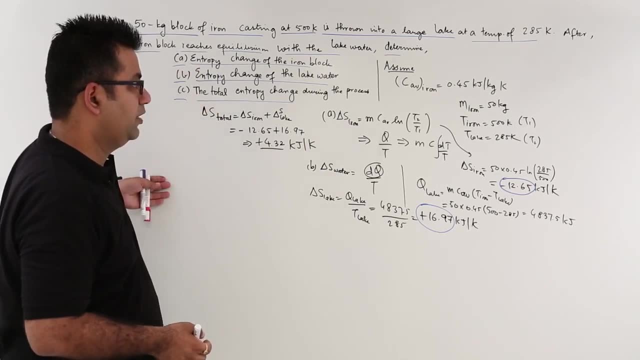 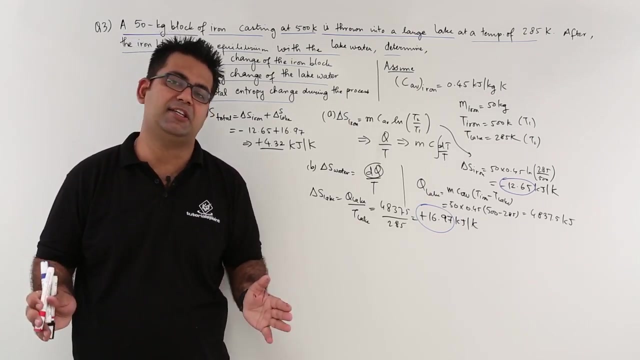 which gives rise to plus 4.7 kilo joule per kelvin. So this is how we attempt a question like this very, very simple to understand. so i hope by now you have understood the entire section of second law and a very important section.